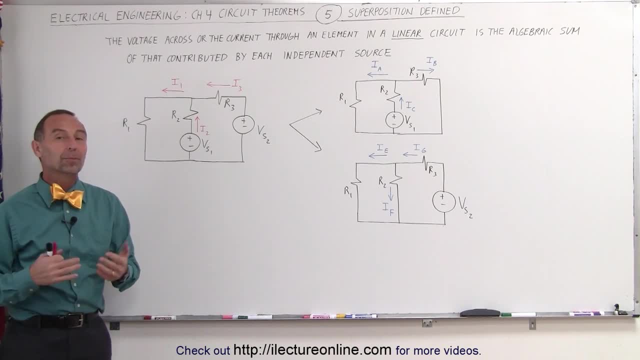 Welcome to ElectronLime. Now let's talk about superposition. What is it? How is it defined? Well, in words, we can define the superposition as the following: The voltage across or the current through an element in a linear circuit. and here's, a linear circuit has nothing but linear elements. 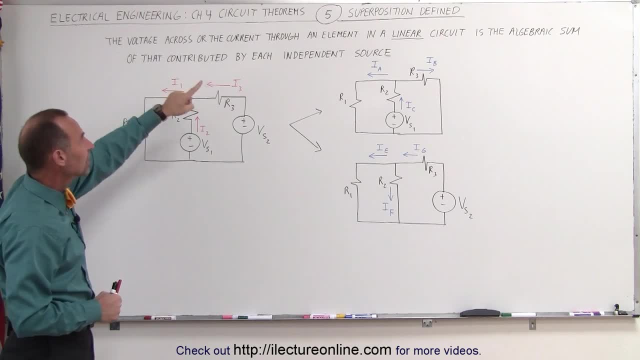 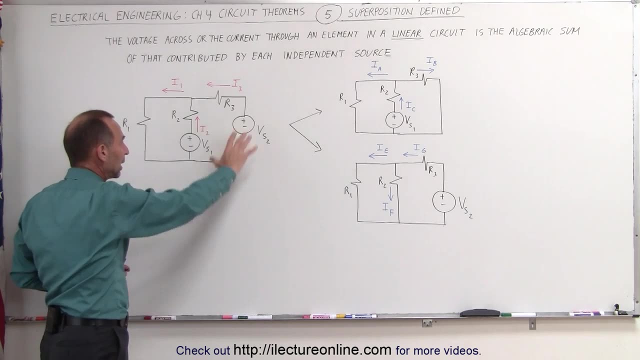 It is the algebraic sum of that contributed by each independent source. Notice, in this case there's two independent sources. They work independently of one another. They are situated inside a linear circuit. The linear circuit has three linear elements, three resistors. 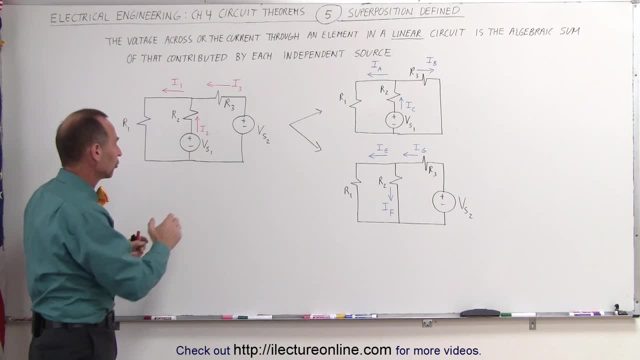 and we recognize that because of those two sources, those two voltage sources, there will be three currents in each of the three meshes or in each of the three branches. If we now separate the two sources, we write the circuit like this, and this is the practical. 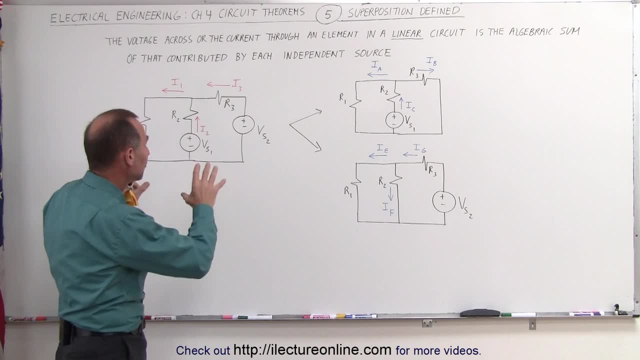 aspect of this whole concept of superposition. If we draw the circuit with any of the three resistors, we have three resistors. If we draw the circuit with any of the three resistors, we have three resistors. If we draw the circuit with any of the three resistors, 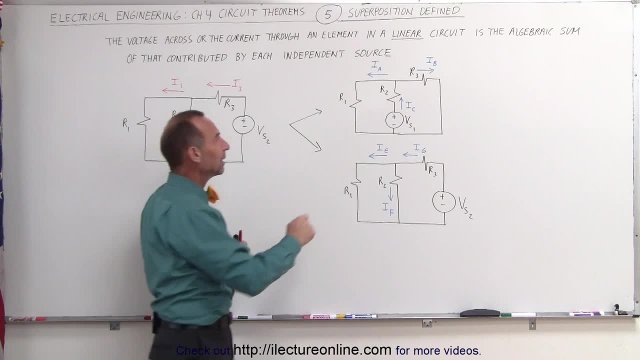 each source separately, like that, and then we calculate the currents through each of the three branches, and then we do it again with the second source and we find the current through each of the three branches solely due to the first source and solely due to the second source. We then know: 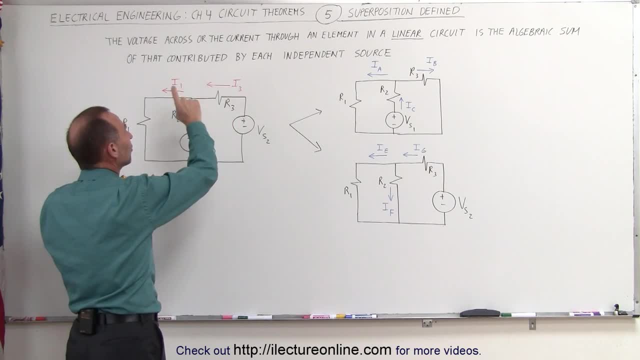 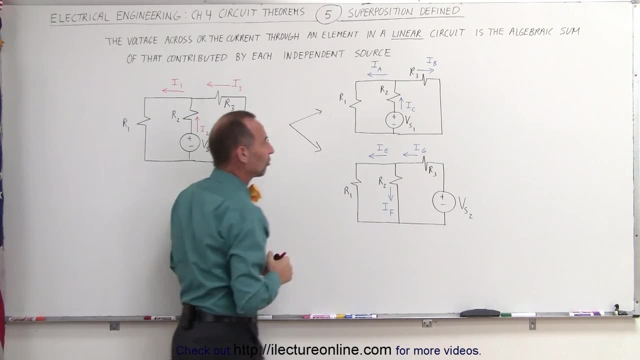 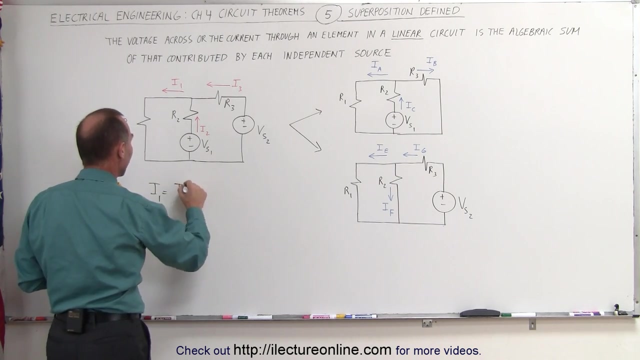 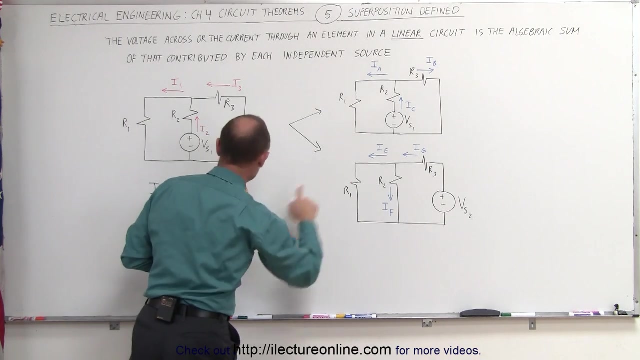 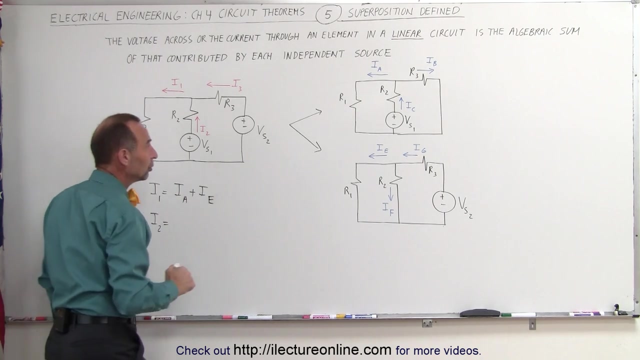 that each of the currents with the two sources present can simply be calculated by algebraically adding the currents found when we do the independent sources like this: With other words, we can say that I1 is simply the algebraic sum of Ia plus Ib and we can say that I2 is equal to the algebraic 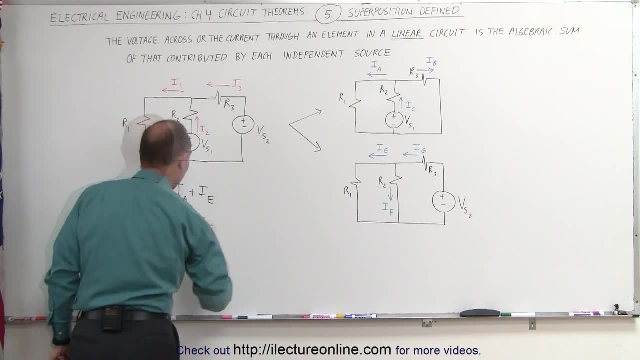 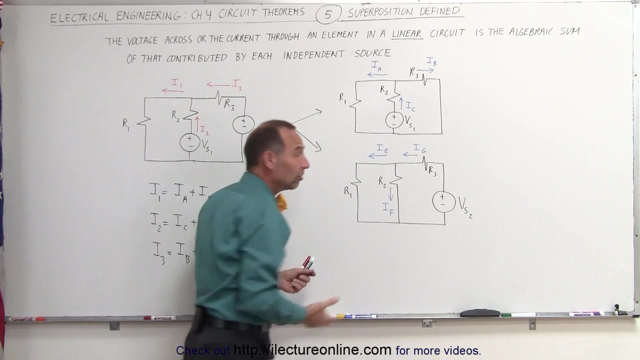 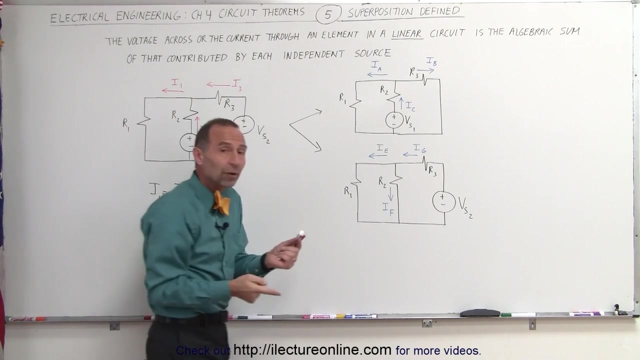 sum of Ic and If, and we can say that I3 is equal to the algebraic sum of Ib plus Ig. Now notice: even though Ib and Ig are in opposite directions, the algebraic sum will still add up to I3.. Also notice that Ic and If are in opposite directions. Again, I2 is simply. 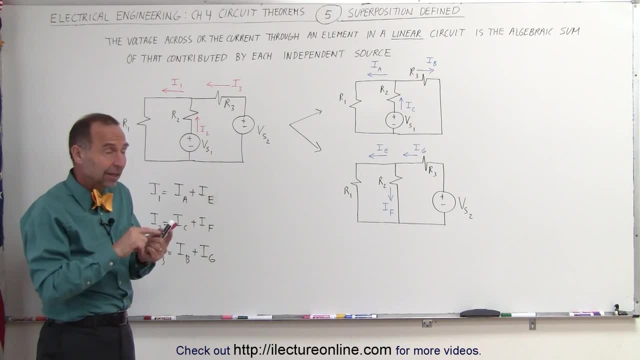 the algebraic sum of Ic, and If so they're in opposite directions- means that one must be subtracted from the other, and the sum of that will still be, or the difference, if you want to call it that- will still be equal to I2.. 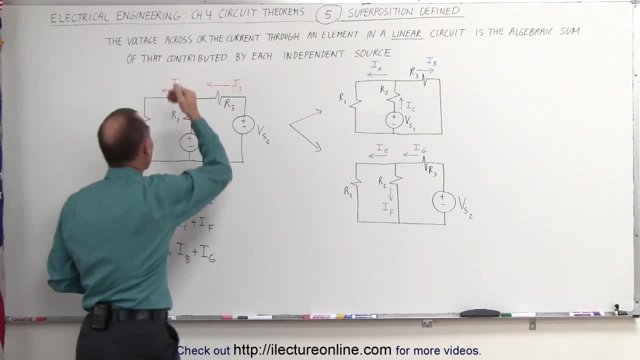 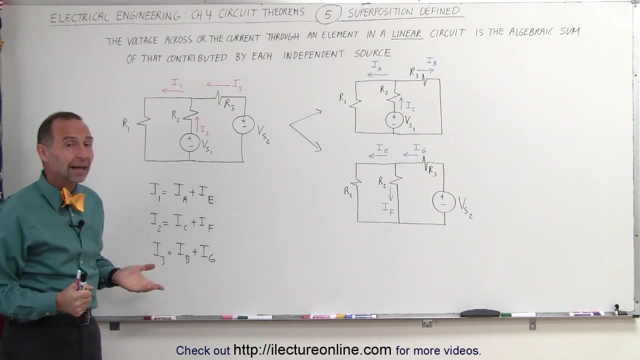 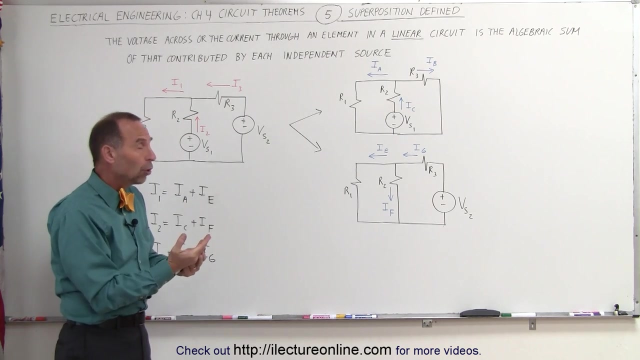 And here you can say that Ia and Ie together will add up to I1. That is really nice. That is one of the methods we can use when we have multiple sources inside a circuit like that. We could solve the circuit by separating it, having each source as a single source in the circuit. calculate all. 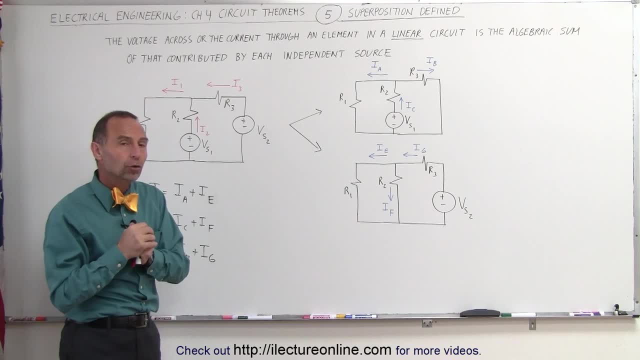 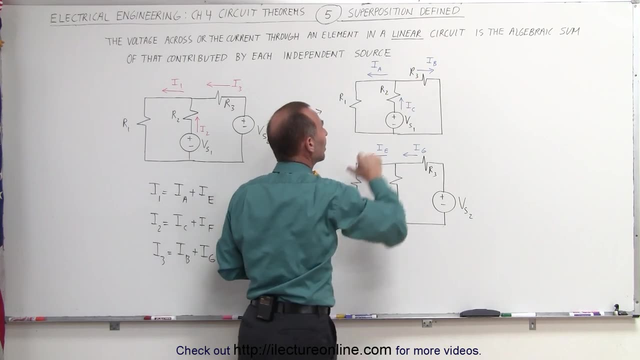 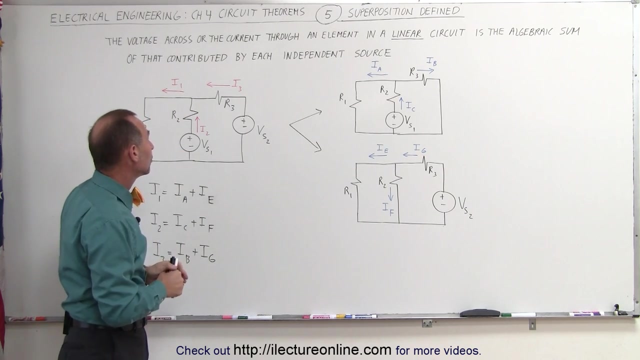 the currents in each of the branches and then simply add up all those currents. Also, if we calculate the voltages at the nodes or if we calculate the voltages across each of the resistors in the circuit, we can again find the total voltage across each of the resistors and the total 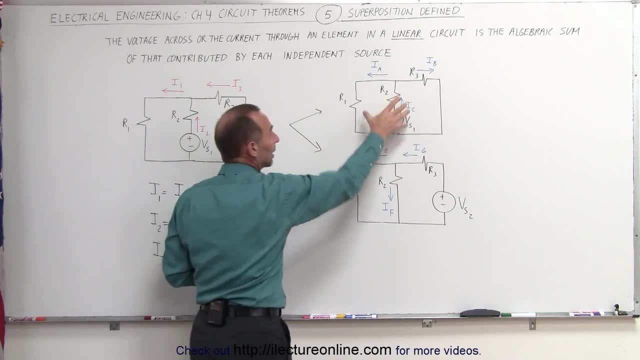 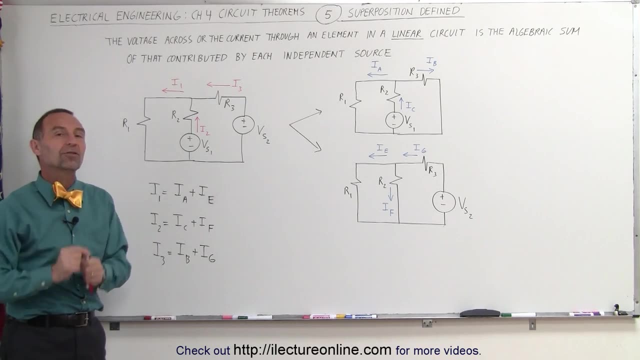 voltage at each node by simply calculating it separately, like this, and then algebraically adding them together. So it works for currents as it does for voltages at the nodes and voltages across the elements. It's a really neat, neat method to use and if you really have trouble, 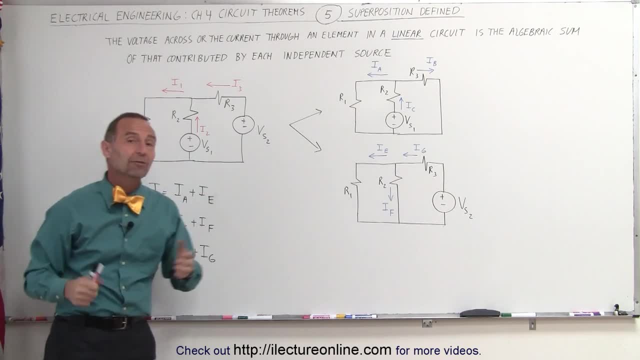 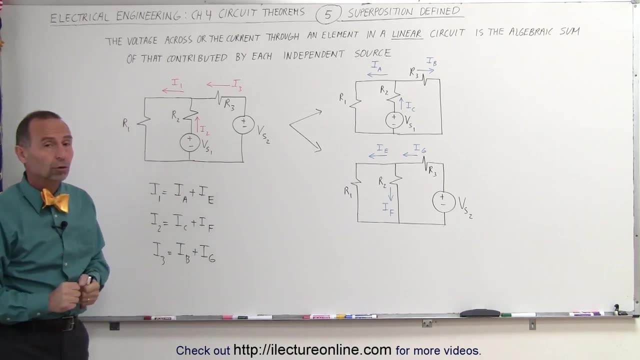 finding it this way. it's easier then to go ahead and separate it and find it that way. Or what you could do is, let's say you used current current and you could do that by separating it, and then supercross laws or rules to calculate the voltages and the currents, or use Thevenin's. 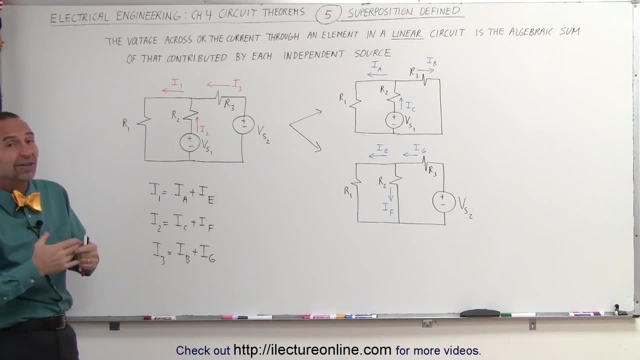 rules or Norton's rules and you're not sure if you did it correctly. you can always do it in a secondary method, like the superposition method: separating the sources, calculating the currents and the voltages independently, adding them together and see if you get the 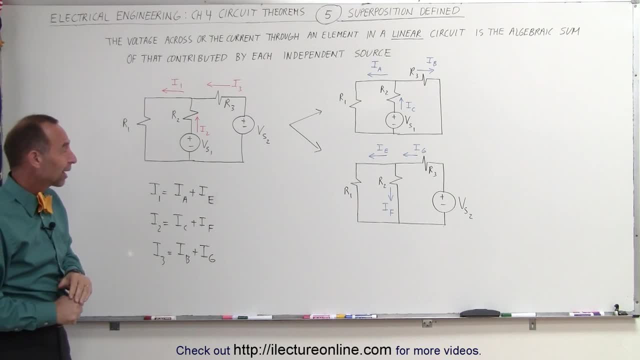 same answer. I do that sometimes just to make sure I did things correctly, But it's a very good technique and we'll show you some examples of how to actually use the technique of superposition. Subtitles by the Amaraorg community.